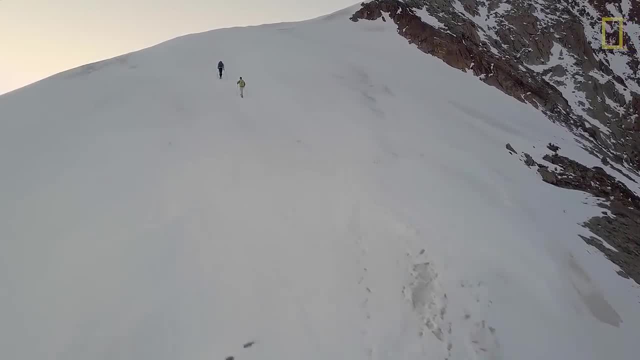 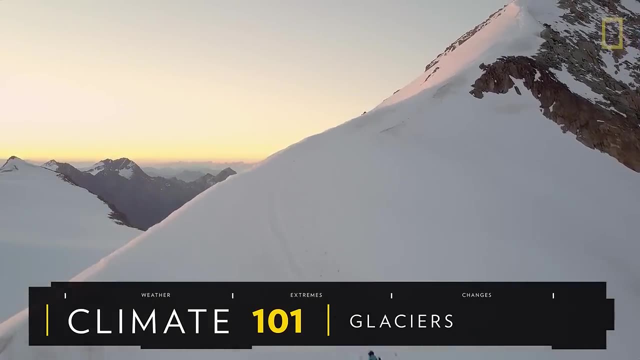 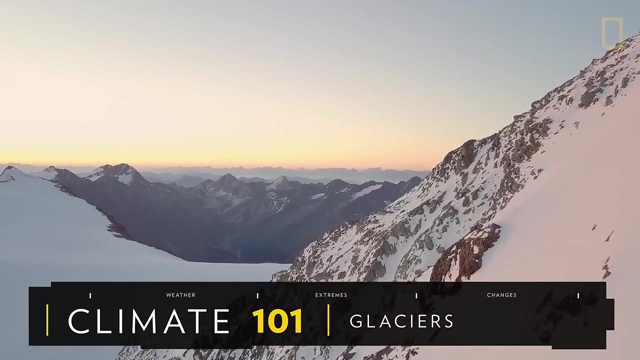 Glaciers have been shaping our world for millions of years, But as climate change warms the planet, glaciers are disappearing, not only altering the landscapes they leave behind, but changing our oceans, weather and life on Earth as we know it. 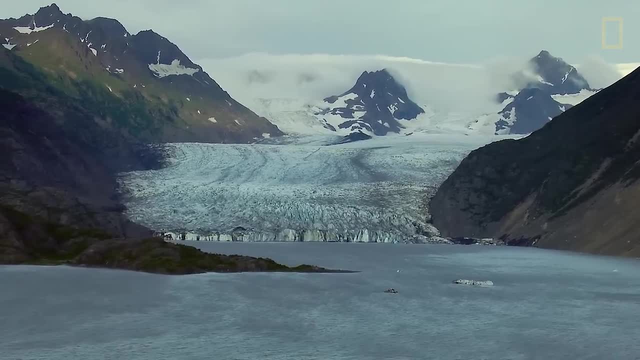 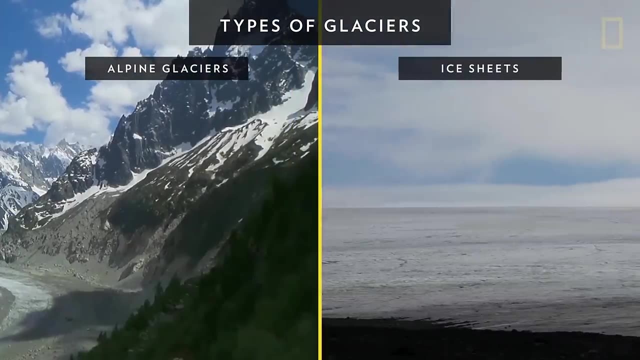 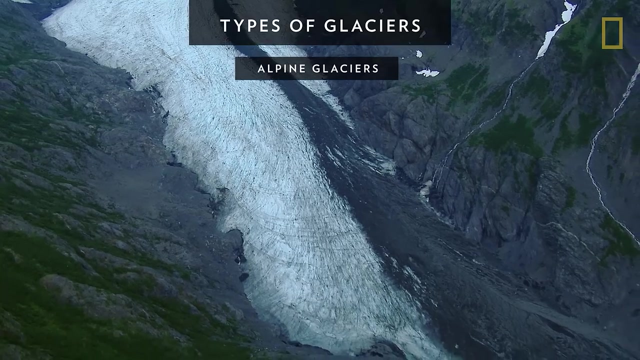 A glacier is a huge mass of ice that moves slowly over land. Glaciers can be classified into two general groups: alpine glaciers and ice sheets. Alpine glaciers form on mountainsides and move downward through valleys. Sometimes they create valleys by pushing dirt, soil and other materials out of their way. 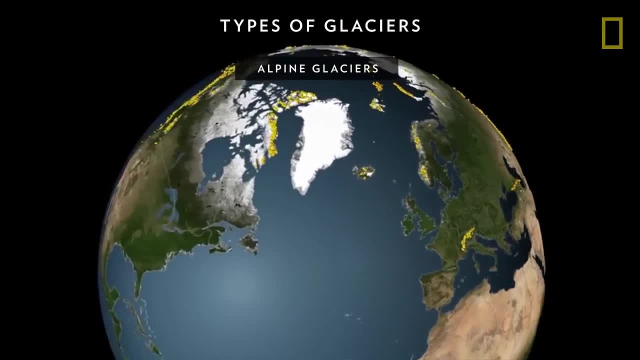 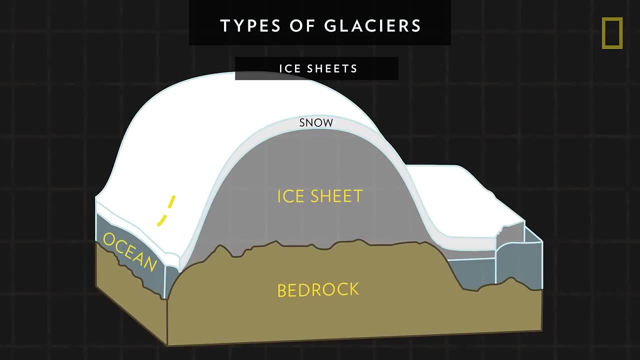 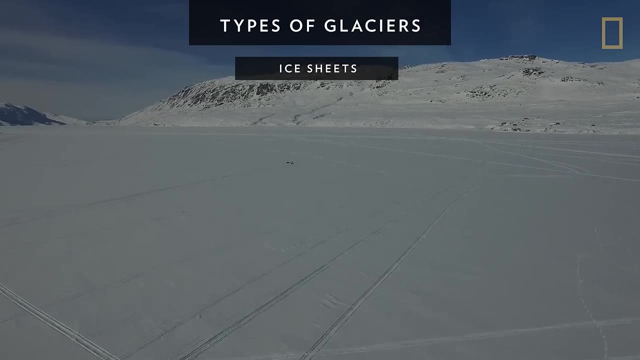 These glaciers are found on every continent except Australia. Ice sheets, unlike alpine glaciers, are not limited to mountainous areas. They form boulders, They have broad domes and spread out from their centers in all directions. As ice sheets spread, they cover everything around them with a thick blanket of ice, including 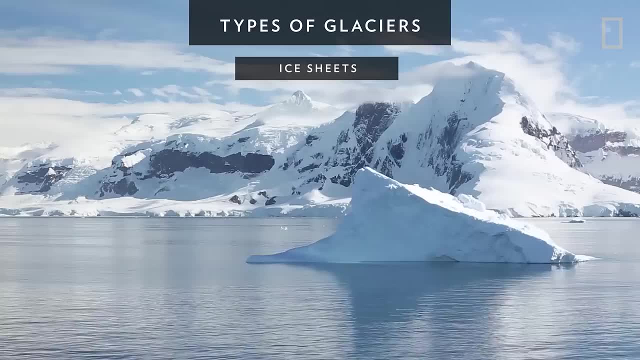 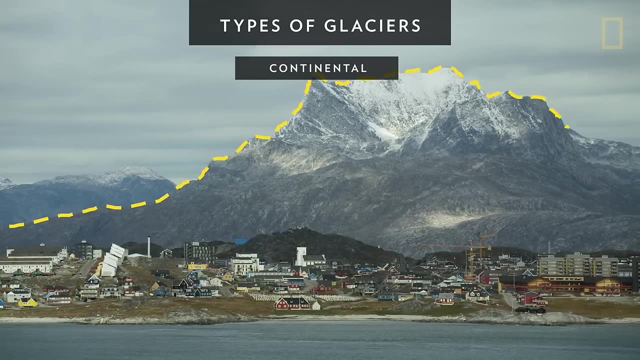 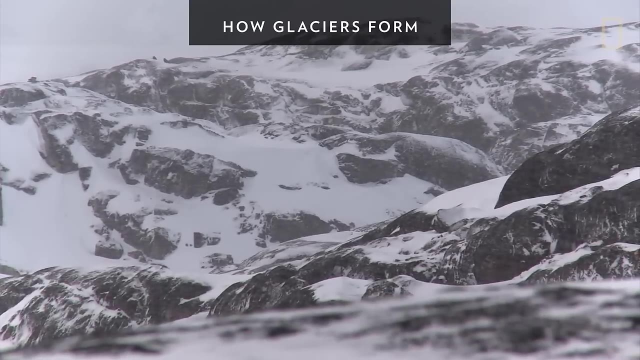 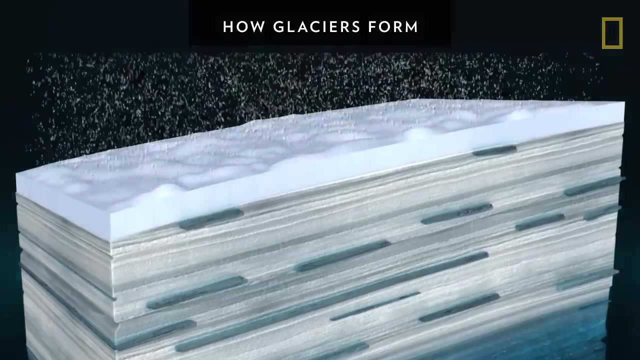 valleys, plains and even entire mountains. The largest ice sheets are called continental glaciers. They cover vast areas, including most of Antarctica and the island of Greenland. Glaciers can form over years when more snow piles up than melts. Soon after falling, the snow begins to become denser and more tightly packed. 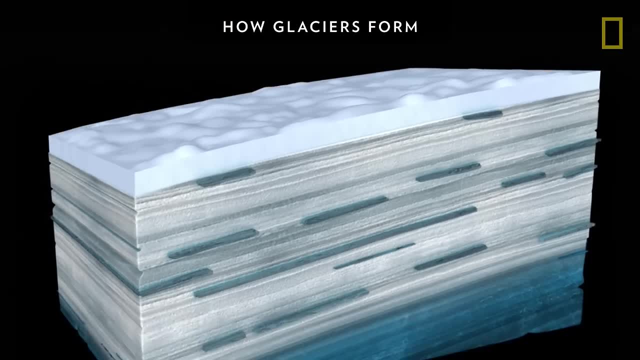 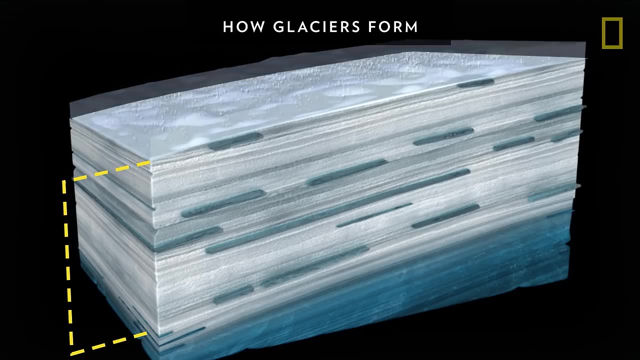 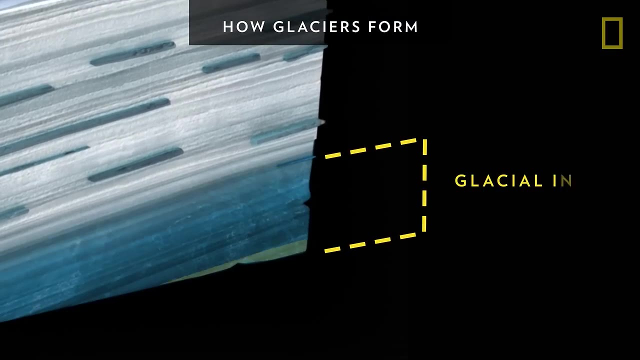 When new snow falls and buries the previous year's snow, the bottom layer becomes even more compressed. The dense, grainy ice that has survived one year's melt cycle is called fern. When the ice grows thick enough, the fern grains fuse into a huge mass called glacial. 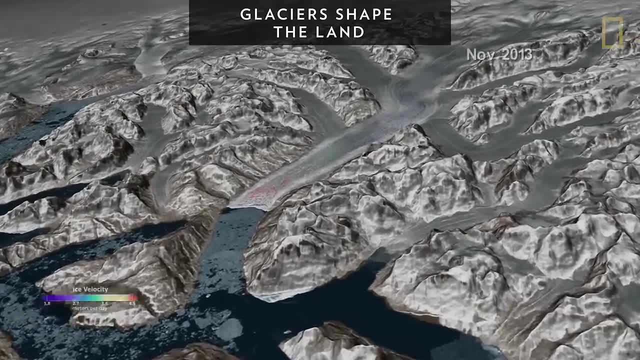 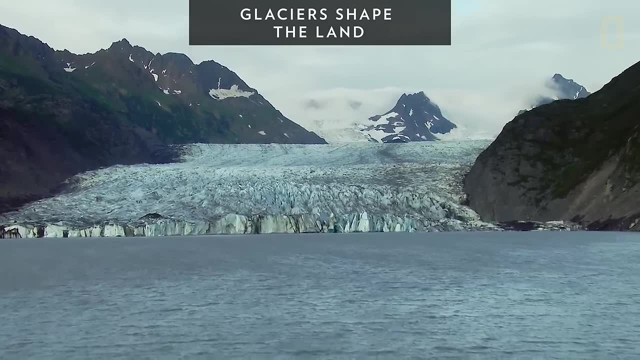 ice. When the ice grows thick enough, the fern grains fuse into a huge mass called glacial ice. Glaciers can move under its own weight through a process called compression melting. As they move, glaciers erode or wear away the land beneath and around them. 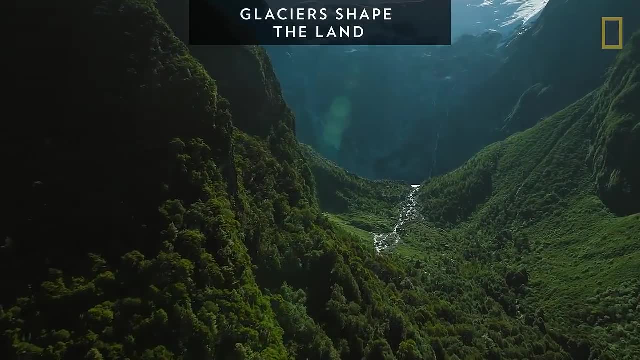 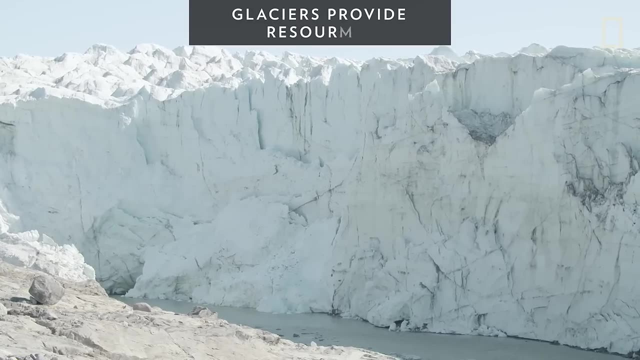 When glaciers began their latest retreat less than 20,000 years ago, they left behind many landscape features, such as lakes, valleys and mountains. Glaciers provide people with many useful resources. Glacial till provides fertile soil for growing crops.